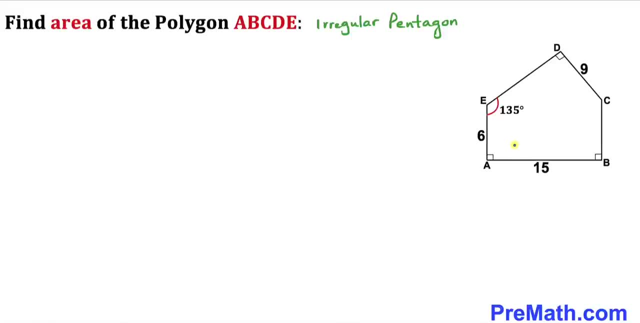 Welcome to PreMath. In this video, we have got this five-sided irregular polygon, As you can see in this diagram, such that it's given side lengths are 6,, 15 and 9 units and, moreover, these angles are 90 degree each and this angle is 135. 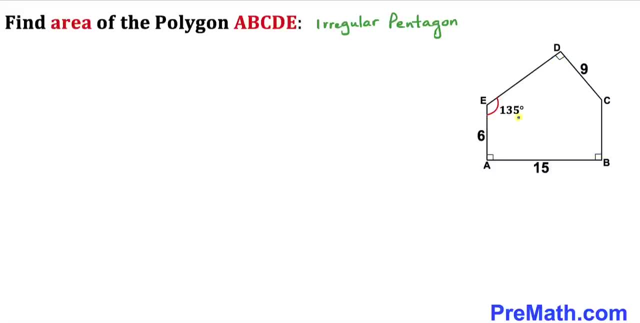 degrees and, by the way, such kind of polygon is called an irregular pentagon. Now we are going to calculate the area of this polygon, ABCDE. Please don't forget to give a thumbs up and subscribe to my channel. Let me make it very clear that this figure may not be 100% true to the scale. 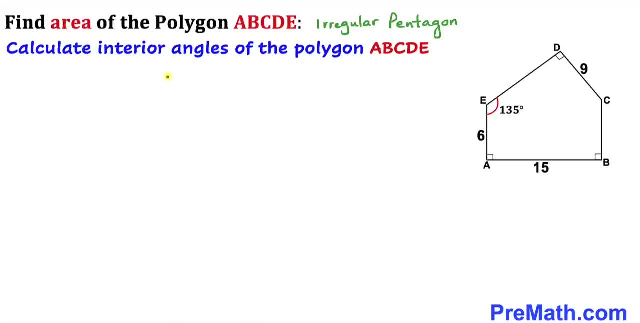 Go ahead and get started with the solution, and here's our very first step. let's go ahead and calculate the interior angles of this polygon, ABCDE, and we know that this angle is 90 degrees. this angle is 90 degrees. this angle is 90 degrees. 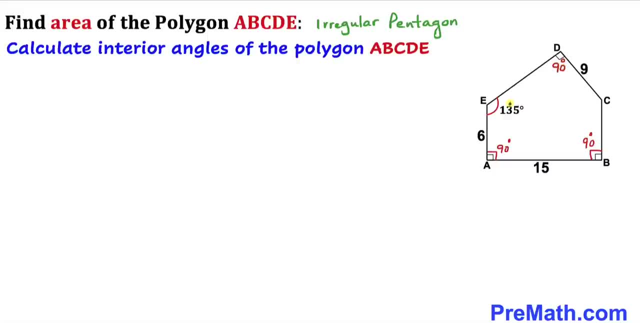 degrees as well, and this angle is 135 degrees. so this is the only angle that we need to calculate. now let's recall the interior angle sum formula. interior sum equals to n minus 2 times 180 degrees, where n is the number of polygon sides, since we are dealing with the Pentagon, so n equals to 5 in our case. 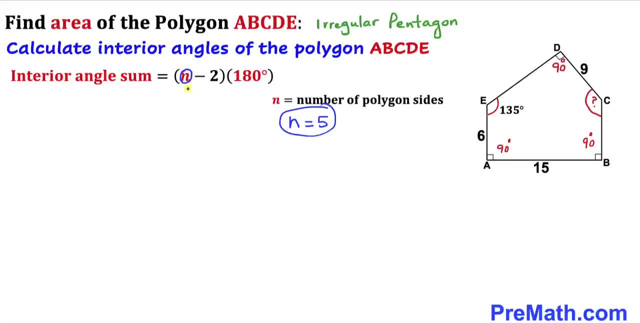 therefore I am going to replace this n by simply 5, so therefore we can write 5 minus 2 times 180 degrees. so thus, if we simplify, our interior angle, sum turns out to be a 540 degrees. so therefore I wrote down these angles: 90 degrees plus 90. 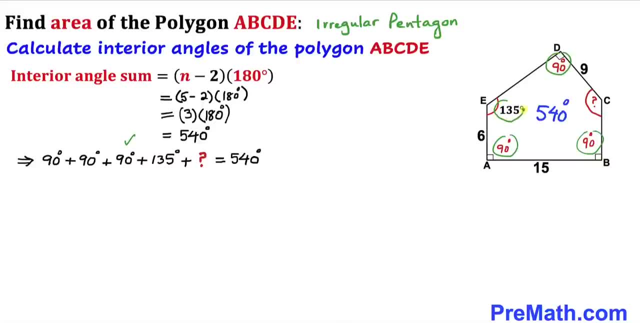 degrees, plus 90 degrees, plus 135 degrees, and then this plus unknown angle on the left hand side, and it must be equal to the total angle. sum is 540 degrees and if we simplify everything, our unknown angle turns out to be 135 degrees. so therefore, this angle is 135 degrees. once again, we are dealing with this. 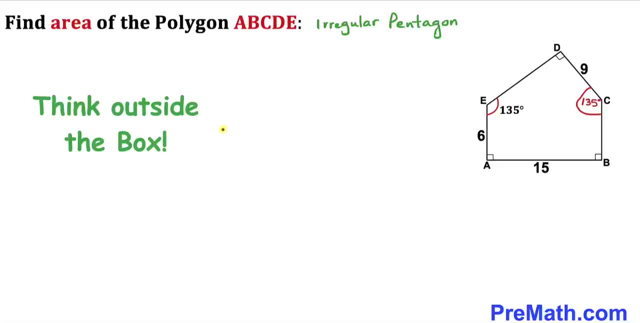 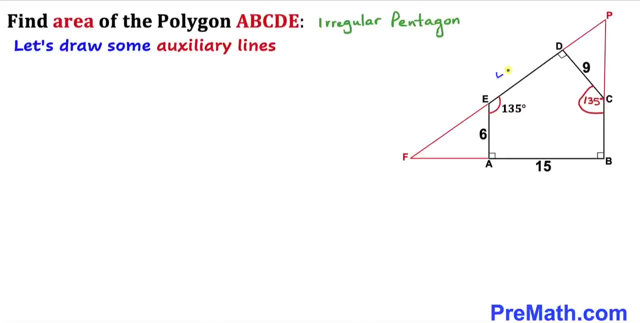 tricky kind of problem, so we're gonna think outside the box. so, therefore, let's go ahead and draw some auxiliary lines, as you can see in this next diagram, and now let's focus on this uh angle over here. the whole this straight angle is 180 degrees, and we know that this angle is 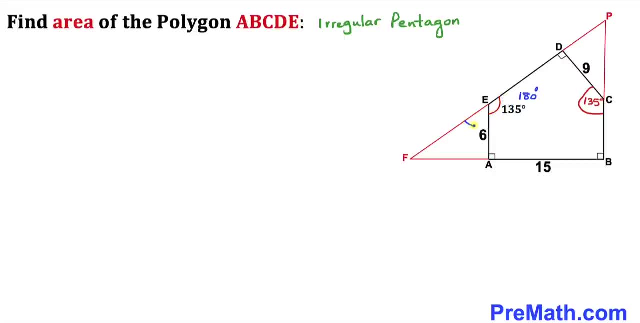 135 degrees, so therefore, this angle is going to be 45 degrees, since the sum of these two angles equals to 180 degrees. and likewise, let's focus on this angle once again. this angle, straight angle- is 180 degrees and this angle is 135 degrees, so therefore, this angle is going. 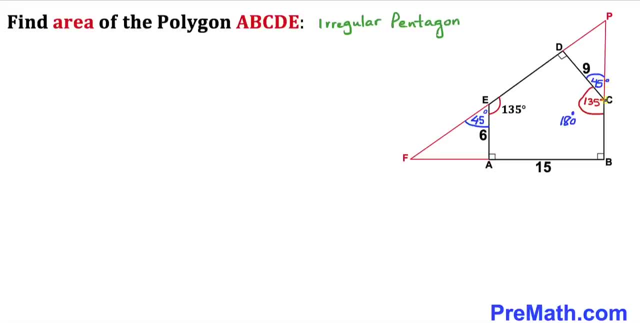 to be 45 degrees as well. and here's our next step. let's focus on this triangle, FAE. we know that this angle is 90 degrees. this angle is 45 degrees, so therefore, this angle has got to be 45 degrees as well, since the sum of these 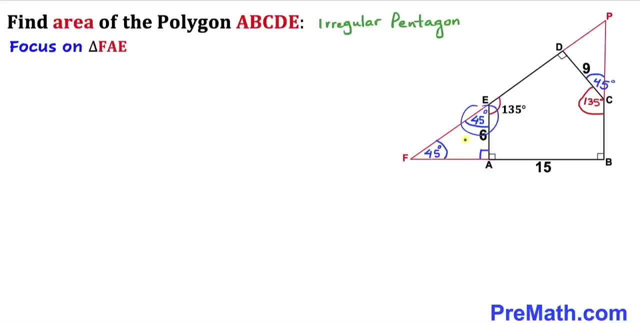 interior angle must be equal to 180 degrees. so therefore, we conclude that this is an isosceles triangle, since this angle equal to this angle. so therefore, this side length is going to be equal to this side length if this side length is 6 units. 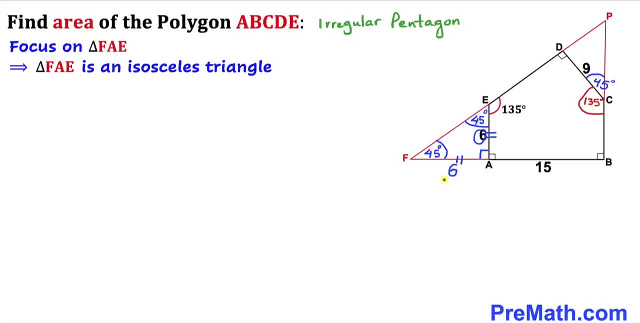 this side length is going to be 6 units as well. so therefore this side length FAE turns out to be 6 units. therefore this whole length FB is going to be sum of these two individual lengths: 6 plus 15. so that is going to be equal to 21 units. 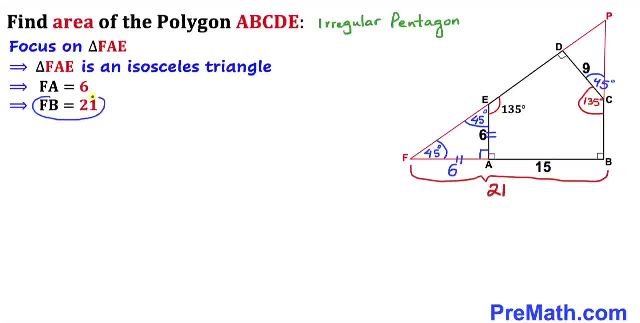 so, therefore, our this length FB turns out to be 21 units. and here's our next step. let's focus on this bigger right triangle fbp. we know, in this triangle, this angle is 90 degrees, this angle is 45 degrees, so therefore, this angle has got to be 45 degrees as well, since the sum of all 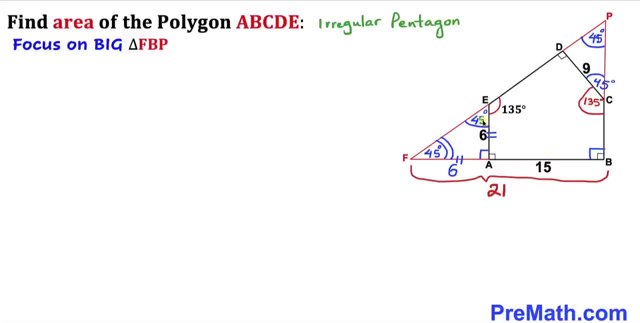 these angles must be 180 degrees or therefore we conclude that the right, this triangle, FPP, is an isosceles triangle, since this angle equals to this angle. that means this side length must be equal to this side length, and we know that this side length is 21 units. so therefore, this side length is going to 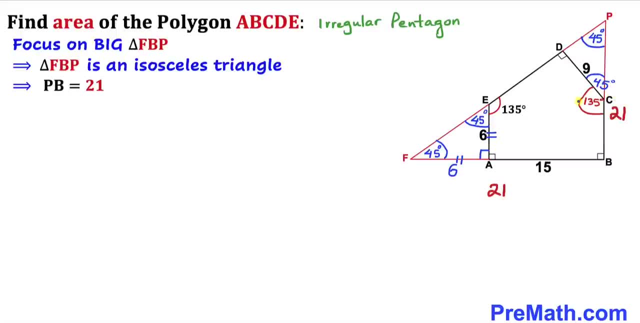 be 21 units as well. therefore, this side length BP turns out to be 21 units. and here's our next step. let's focus on this triangle, PDC, and we can see that this is an isosceles triangle, since this angle and this angle, they are 45. 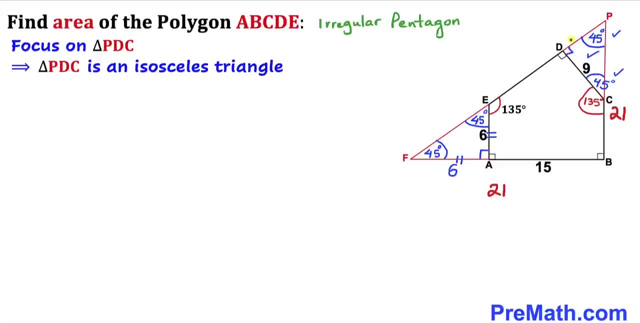 degrees each, and this is our 90 degree angle. so therefore, our this side length is going to be equal to this side length. if this side length is a 9, this has got to be 9 units as well. so therefore, our side length PD turns out to be 9 units. 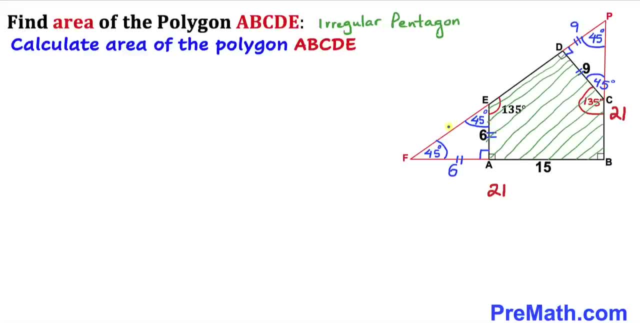 as you can see over here, and in this next step, we are going to calculate the area of this polygon ABCDE, and here's the strategy we're going to be using. area of this polygon ABCDE is going to be equal to the area of this bigger triangle, FPB minus the area of this smaller. 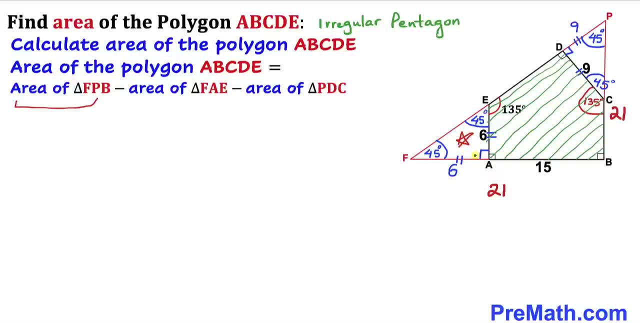 triangle, this one which is FAE, and then minus this triangle, PDC as well. and if I represent the area of this bigger triangle as uppercase a and the area of this smaller triangle FAE as a sub 1, that means this is a sub 1 minus the area of this PDC smaller triangle. I'm going to call the. 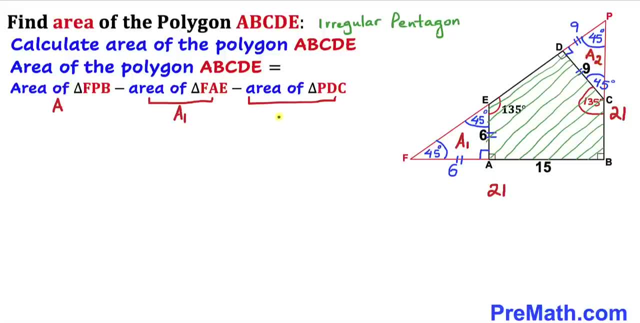 area a sub 2. so this area is a sub 2. so therefore the area of this polyafleet Promised jeder minimal k Ecu rugby 1 fordi gesamte objektiv. Let's check it out. a, b, c, d is going to be a minus a sub 1, minus a sub 2, and here's our next step, let's go ahead. 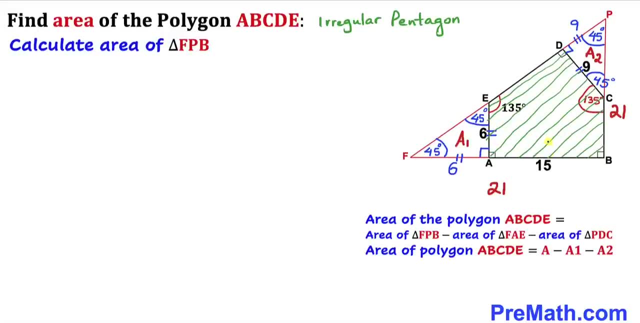 and calculate the area of this big triangle f p b. now, let's recall the area of a triangle. formula area equals to a half time base time height. in our case, our base is 21 and our height is 21 units as well. so, therefore, the area of this triangle f p b is going to be- i'm going to 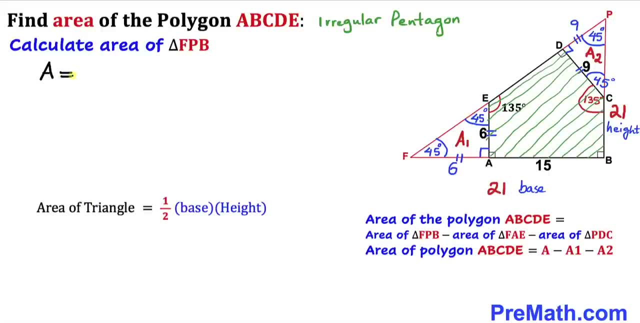 represent it with the uppercase. a equals to a half times 21 times 21 as well. so therefore this area a turns out to be 220.5 square units. and here's our next step. let's go ahead and calculate the area of this big triangle. f p b is going to be a half times. 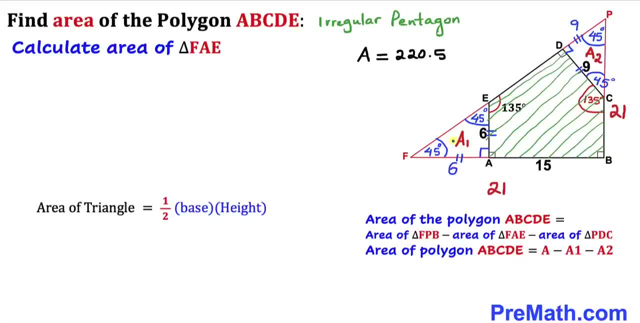 let's go ahead and calculate the area of this smaller triangle, FAE, and once again we're going to be using this formula of the triangle and in our case, our base is 6 and our height is 6 units as well. so, therefore, the area of this triangle FAE- I'm going to represent it by a sub 1- is going to: